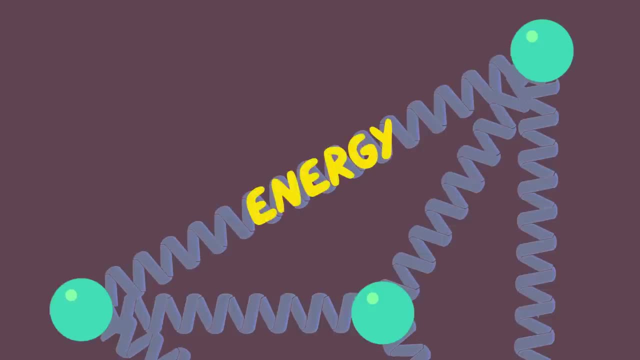 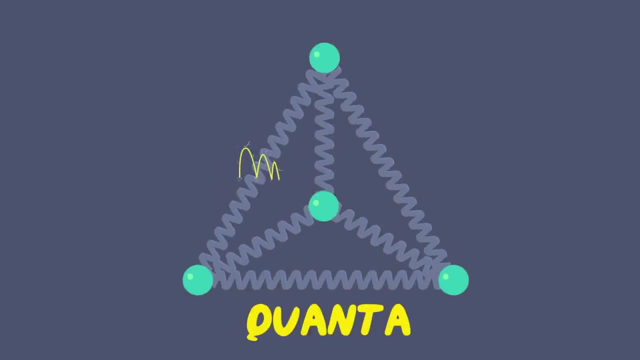 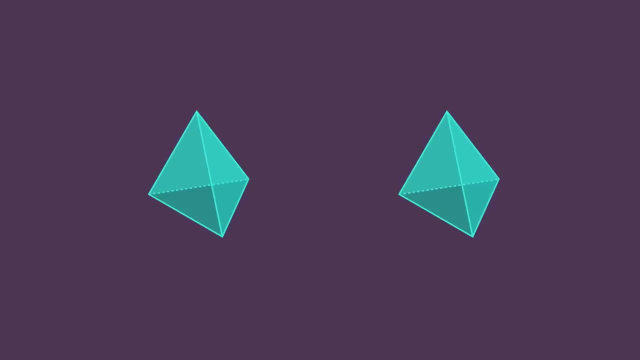 In this model, the energy in each solid is stored in the bonds. Those can be thought of as simple containers which can hold indivisible units of energy, known as quanta. The more energy a solid has, the hotter it is. It turns out that there are numerous ways that the energy 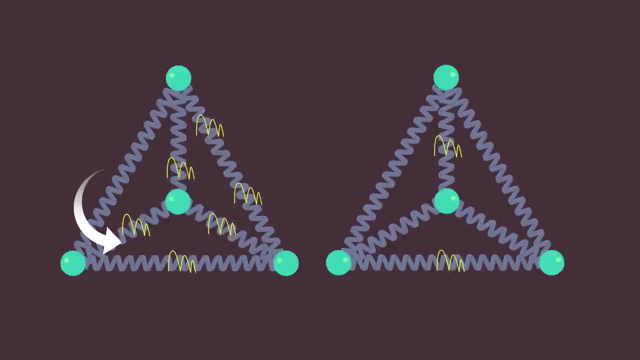 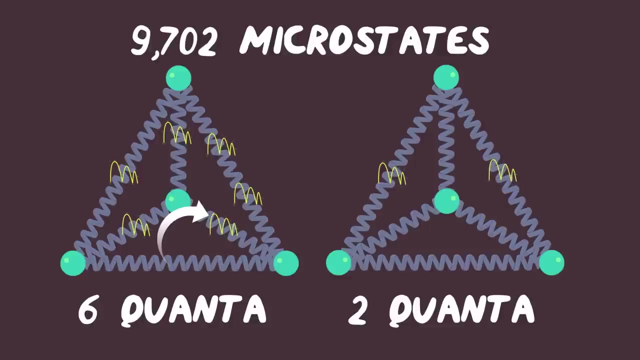 can be distributed in the two solids and still have the same total energy in each. Each of these options is called a microstate, For six quanta of energy in solid A and two in solid B. there are 9,702 microstates. 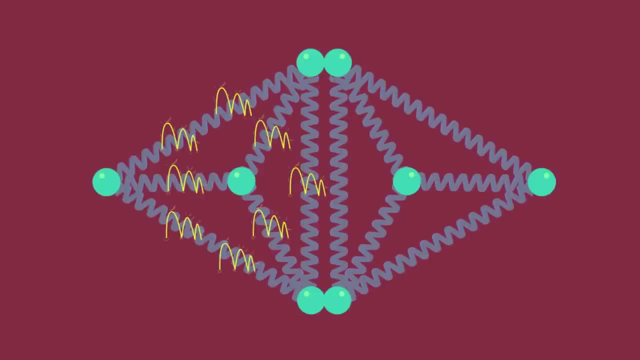 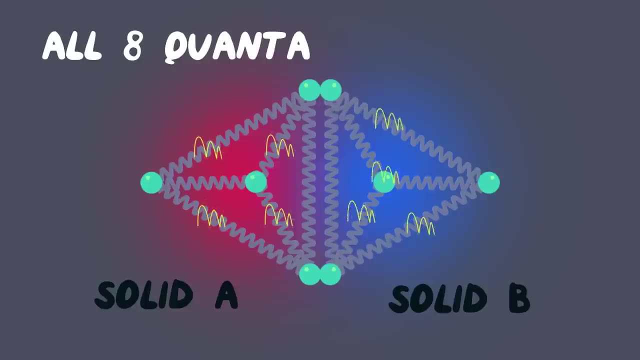 Of course there are other ways our eight quanta of energy can be arranged. For example, all of the energy could be in solid A and none in B, Or half in A and half in B, If we assume that each microstate is equally likely. 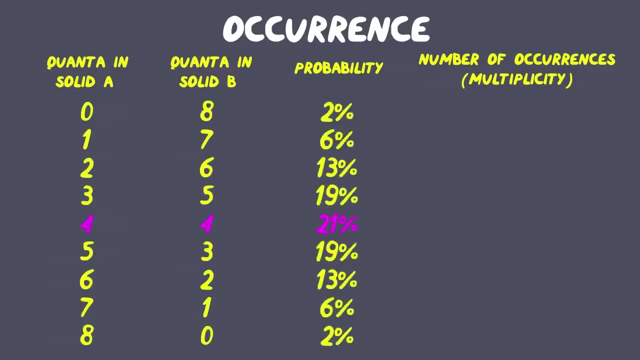 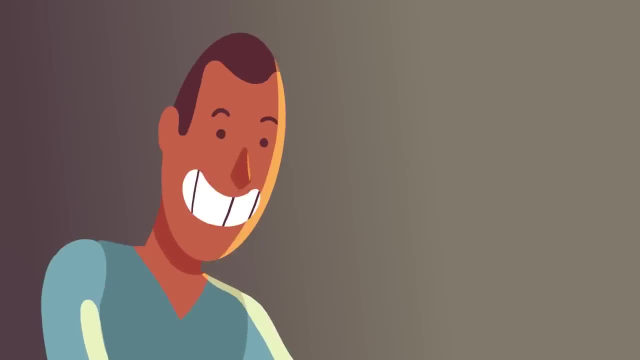 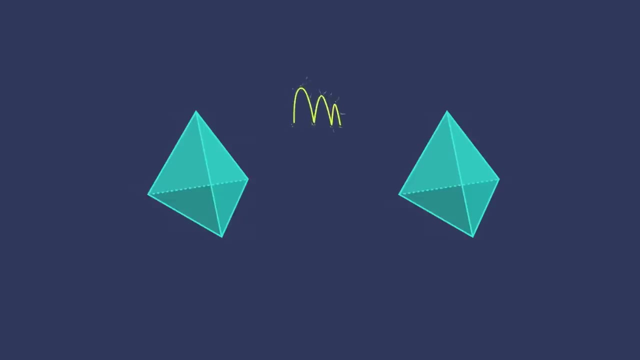 we can see that some of the energy configurations have a higher probability of occurring than others. That's due to their greater number of microstates. Entropy is a direct measure of each energy configuration's probability. What we see is that the energy configuration in which the energy is most spread out between the solids has the highest energy. 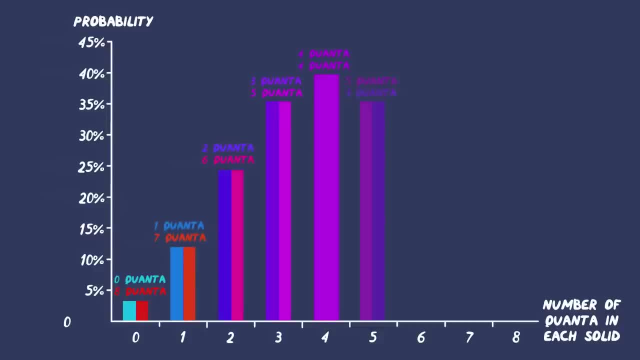 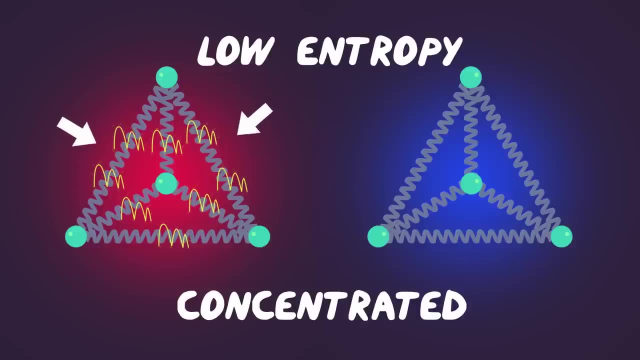 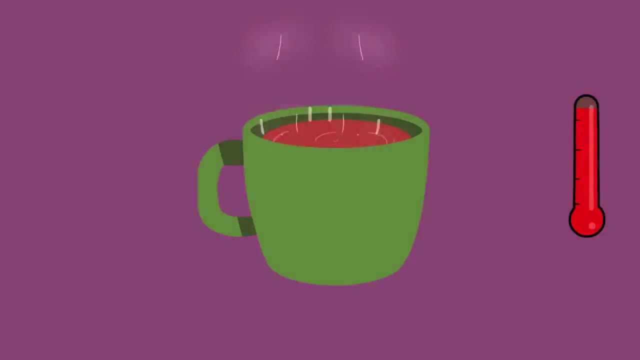 That's entropy. So in a general sense, entropy can be thought of as a measurement of this energy spread. Low entropy means the energy is concentrated. High entropy means it's spread out. To see why entropy is useful for explaining spontaneous processes like hot objects cooling down. 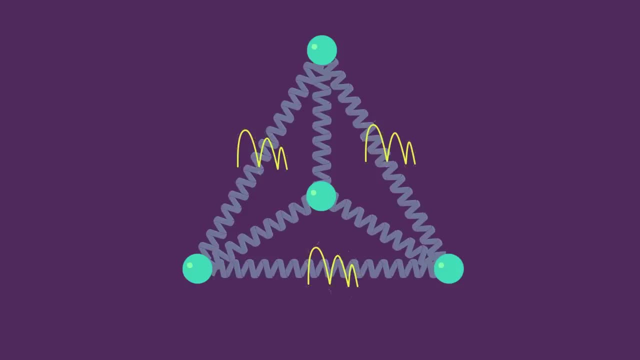 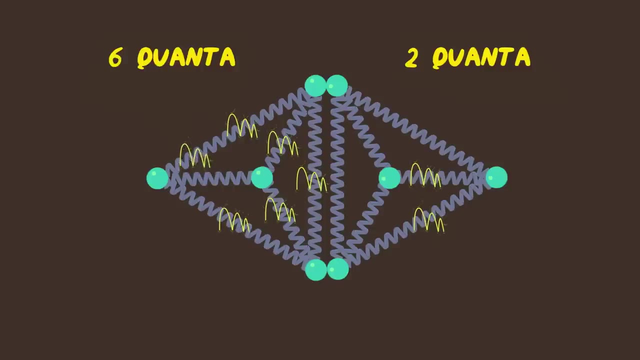 we need to look at a dynamic system where the energy moves. In reality, energy doesn't stay put. It continuously moves between neighboring bonds. As the energy moves, the energy configuration can change Because of the distribution of microstates. there's a 21% chance that the system will later be in the configuration. 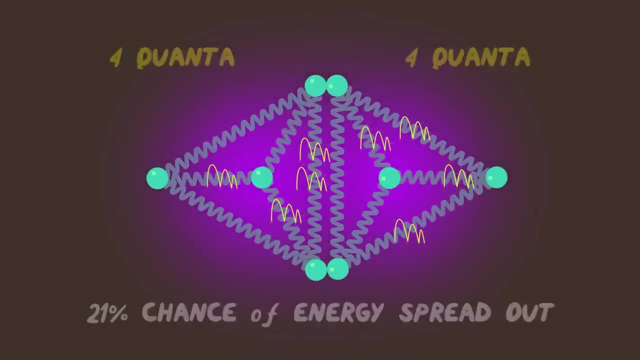 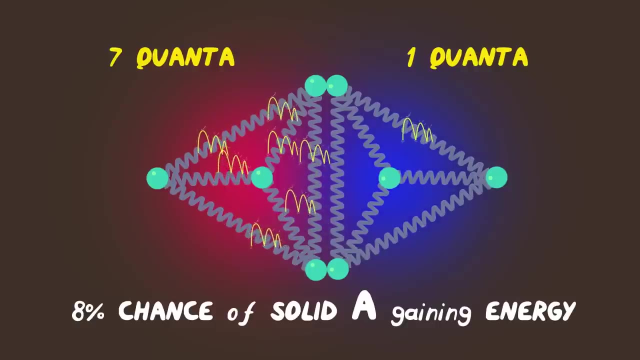 in which the energy is maximally spread out, There's a 13% chance that it'll return to its starting point and an 8% chance that A will actually gain energy. Again, we see that because there are more ways to have dispersed energy.